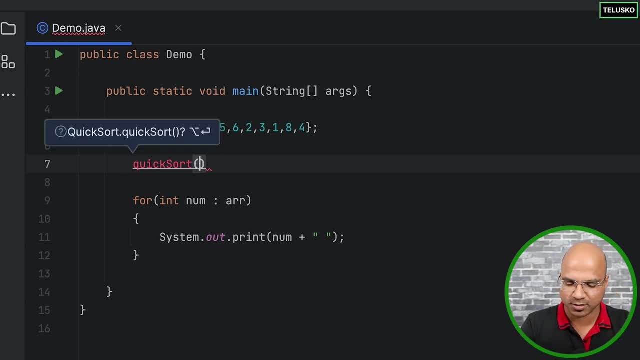 Which will take three parameters. Now, what are the three parameters? The first one is the array itself, on which you want to perform the operation. Next is the starting point and the ending point of each section. Example: if you start, it will be the entire array, but remember when we have to break it down, So that is your each section. Okay, so we have to specify the low and then you have to specify the high. Now, in this case, what is low? So low is zero and the high is basically the array. 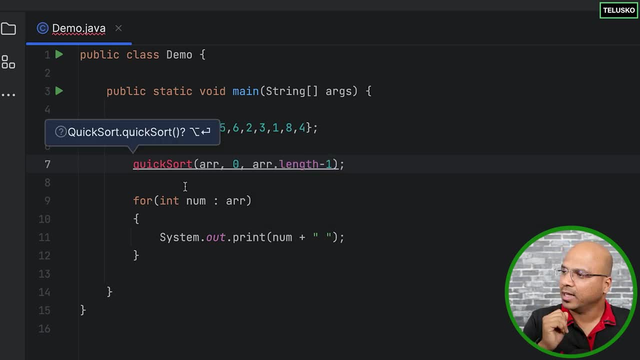 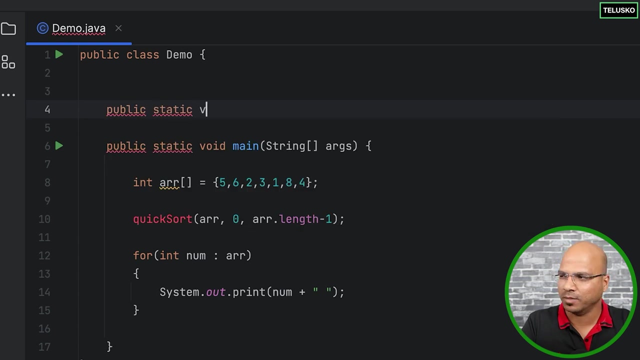 dot length minus one. Right, that's the value you have to send Now. basically, we don't have this function, So we can just right click here and say, okay, I want the IDE to create this method for me, Maybe just using some inbuilt methods. Okay, let's create our own. So what I will do here is I will create a method called public. I don't want to get the object, so I will say static, void, quick sort, and it will take these three values. So first it will take an int array, In fact one of the syntax of array. you can write it on this side because it will make much more sense. You got 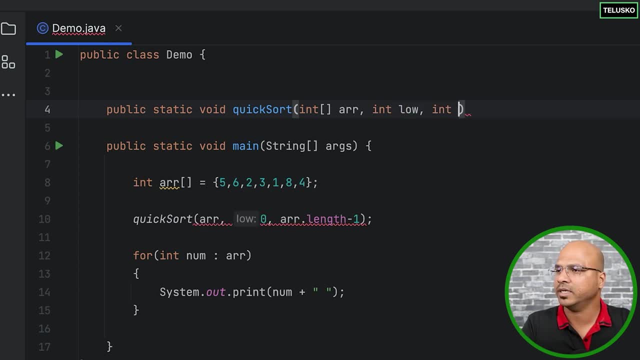 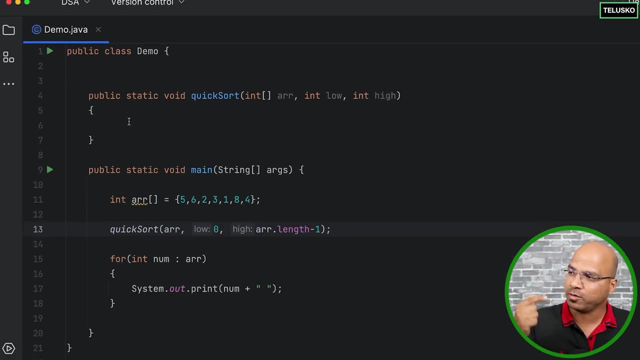 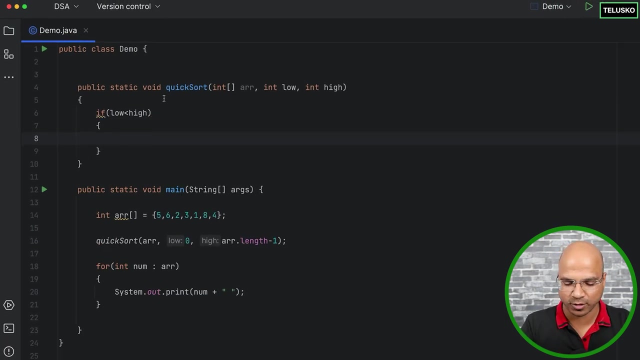 array, and then you got int low, then you got int high. So these are the variables you need and then you can start performing the operation. So basically, from the main, you're calling quick sort only once, but quick sort will be calling itself. Okay, but based on what? Now? basically, I want quick sort to call itself only till when your low is less than high. We don't want it, right? So that's what it makes sense, right? Low should be low, high should be high, and if it is true, then keep calling the quick sort. So I will keep calling the quick sort, but the question is what values I have to pass. Now think about it. 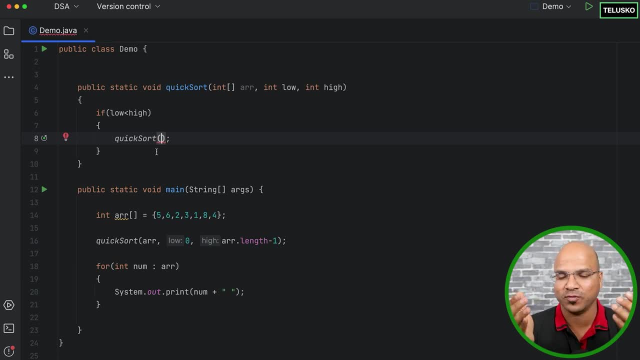 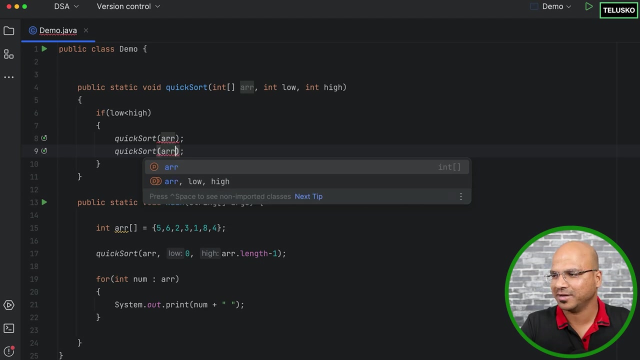 If you have one big array and then you're saying that we'll be breaking this into two parts, So don't you think you have to call quick sort two times for two different arrays. That's right. So you have to call it two times. But the question is: what are the values? For sure, the first variable will be array, because that's what we are sending, right. We have to sort the array. The question is, what will be the low, what will be the high? Because when you divide your array into two parts, what should be the starting point of the second array and the ending point of the second array? That's what you have to mention. But how will you know the starting point? It? 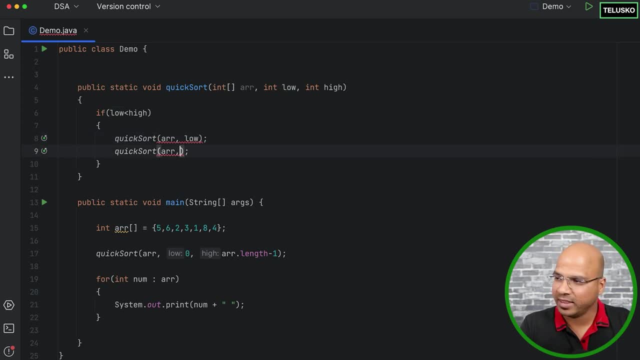 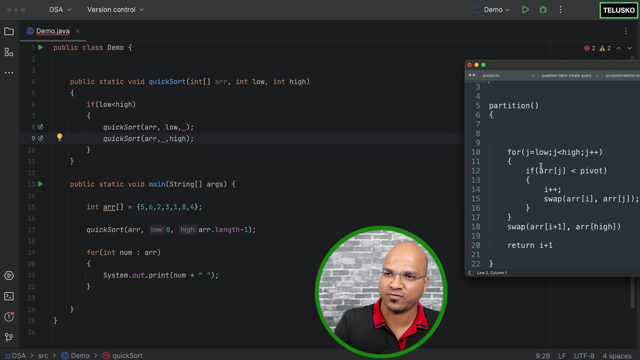 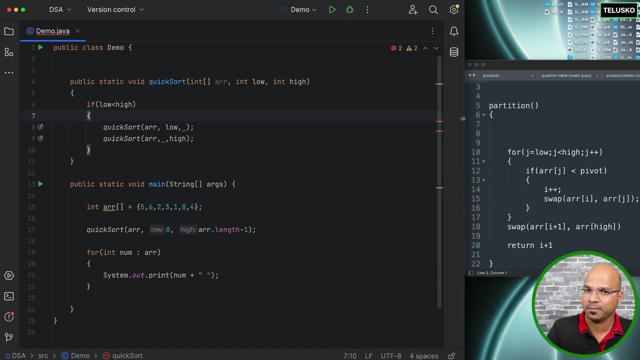 is easy. actually, Here the starting is always low for the first array and the ending is always high for the second array. Even that is solved. The problem is with the ending of the first array and the starting of the second array. That's what we need to find. Now. how do you find this? For this we have to run a partition. So this is the logic which we have to refer to. So what I will do is I will just reduce the array size so that I can see those values. I mean this logic. So this is what we have to implement in the partition. So basically, to get this value, the pivot value, what you will do is you will say int, pi. 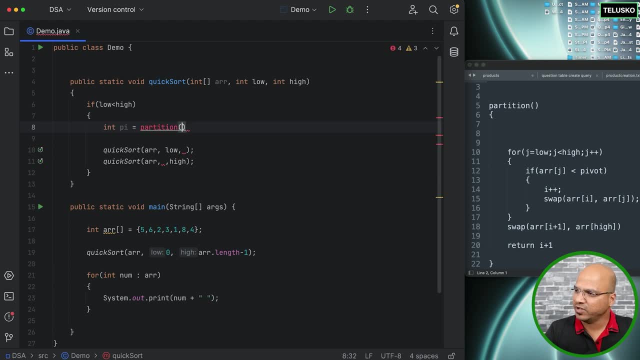 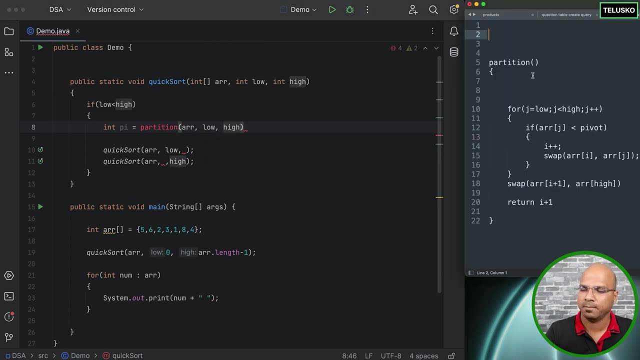 equal to, and you will create a method called partition in which you will pass three values. The same three values: Array, low and high. So basically, in the logic, I have not mentioned it, but we want this value as well, So we need to create this method. So what I will do is I will just go back here: More actions, Create a method. So we got the method. Let's perform an operation on this method. We can make it private, because we are not going to use partition outside this class. So private works. But what should be the logic here? And we have to. 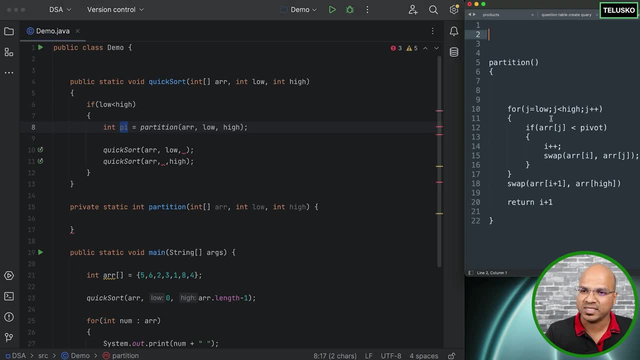 return something. Remember, we have to return the pi value. Okay, So we can write the same logic which we have written here And once you get this pi, you can basically pass the pi. And we don't want to include the pi. So we can say pi minus one, And here we have to pass pi plus one, Because every partition when you create, you don't consider the pi, Pi stays there. You create two parts and then those are your two partitions, But we have to find this pi. That's the main task And for that we have to write this logic which is mentioned here. So we need some variables. The first one is: 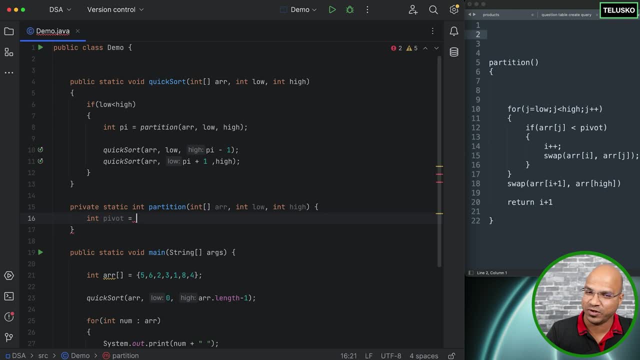 temporary pivot variable And we have to assume pivot for the first time, So the pivot here is always high. So that's the algorithm we are using, But we can pick up the starting value or randomly pick any value that works. So let's say we got pivot high. And then we also need one more variable, which is i. Remember we have to use this i, which we return, So i is basically your low minus one. Remember, if the array starts with zero, the i will be at minus one. Next we need 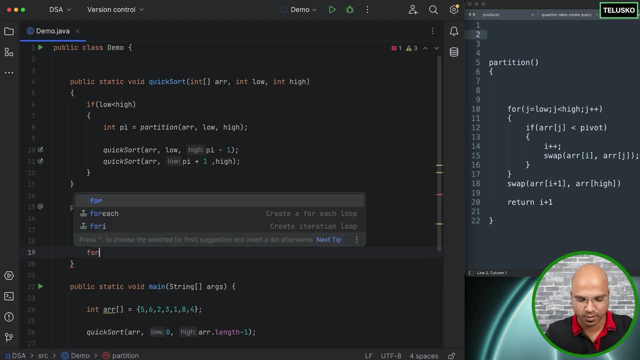 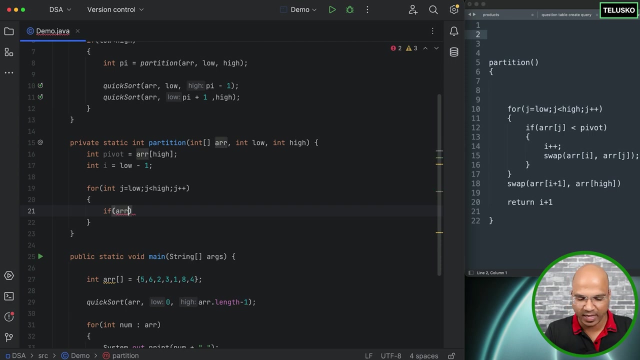 a loop So we can get the entire loop from here. Or maybe you can type So we can say: for int j is equal to zero. In fact, not zero right, It should be always low, Because when you create different partitions, not every partition will start with zero, But they will start with low. So j less than equal to high and j plus plus. I'm just referring to my algorithm which I mentioned here. And then the logic we have to write is: if arr of j, if it is less than pivot, then you 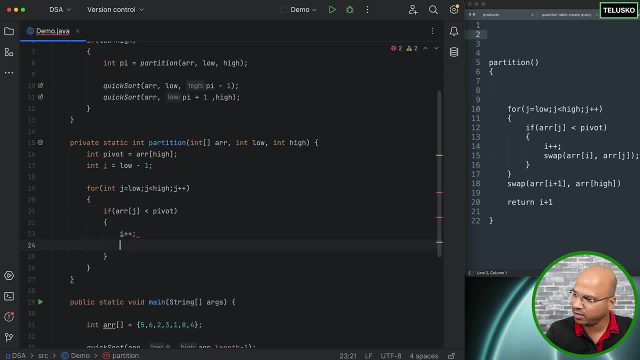 start doing some operation. What operation? First you increment the value of i And then you swap. But how will you swap? We don't have a swap function. Actually, we can create one, But instead of that, what we can also do is we can write the logic So I can say: 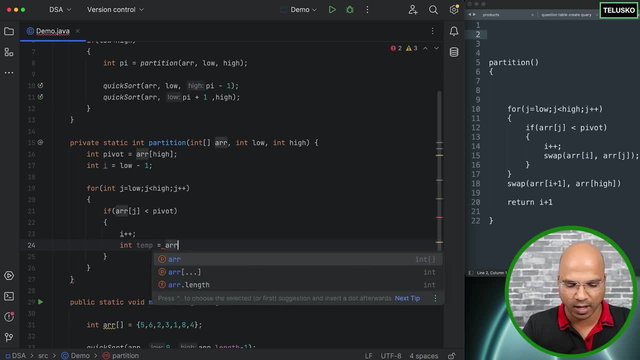 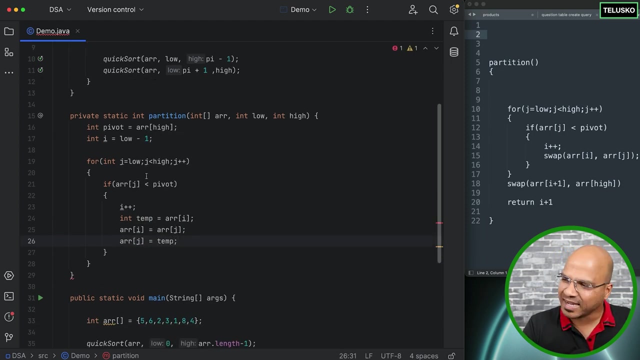 int temp is equal to arr of i, Then arr of i will be replaced by arr of j, And then arr of j will be replaced by the temp. That's the values we have to swap, And that's it. This will run and you will do the partitioning part, But once you complete the for loop. 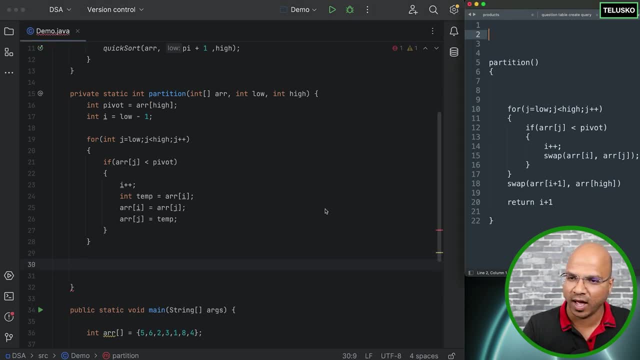 again, we have to swap the value of i plus one with high, So you can actually use the same logic here, Same statements. So I'm not copy pasting, I'm just reusing the code. Sounds better, right? So here we can say: this will be replaced by i plus one And i plus one. 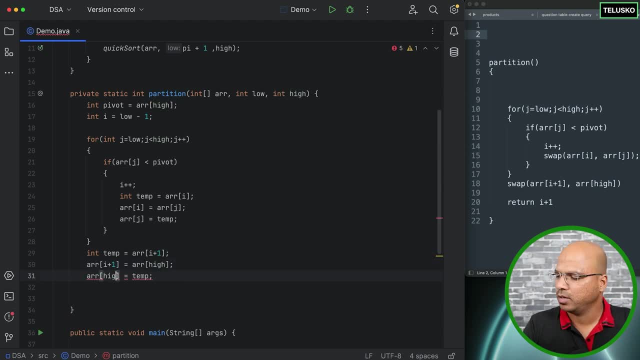 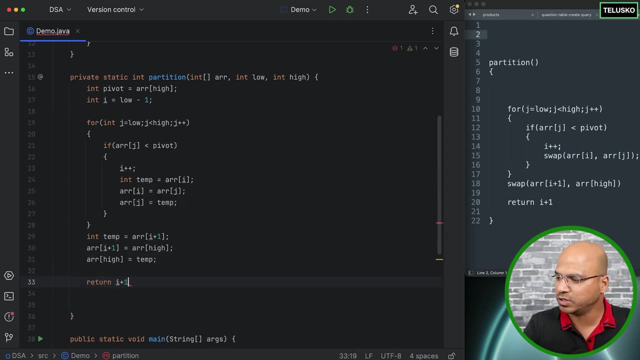 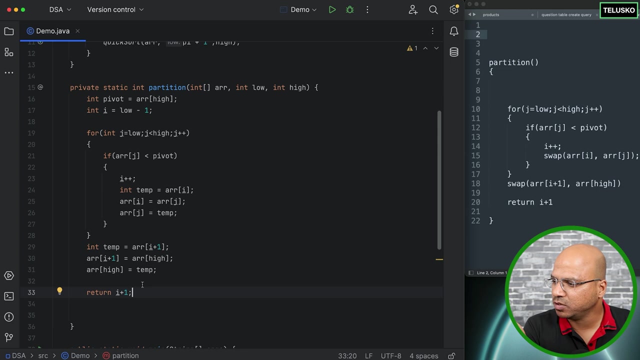 will be replaced by high And this high is going to be replaced by temp Swapping done. At the end we need to return i plus one, because that's what is referring to, the pivot. Okay, Looks like a right logic. We just converted that into here. So by doing the partition, 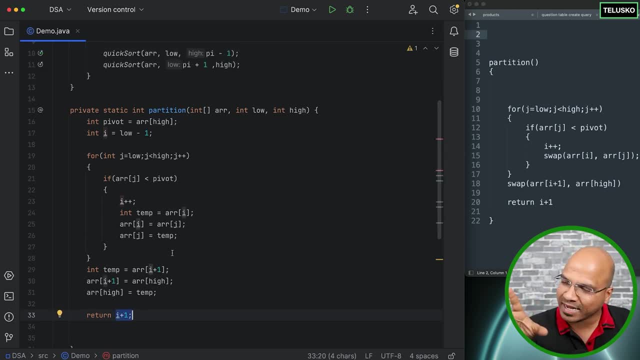 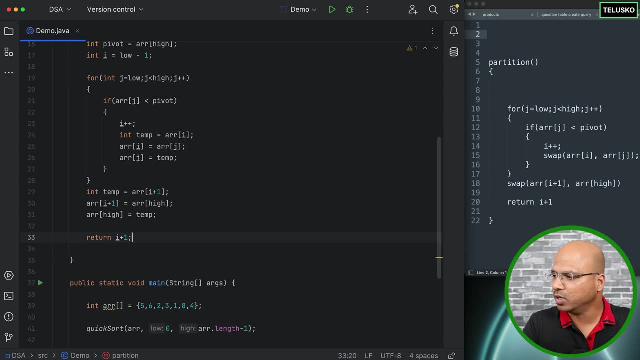 we are saying: replace one. In fact, once you get this algorithm, also try out the same thing which I've done on the board. Okay, Then it will make much more sense. Okay, I hope this will work. What do you think? Let's run and let's see Run. and, yes, Looks like. 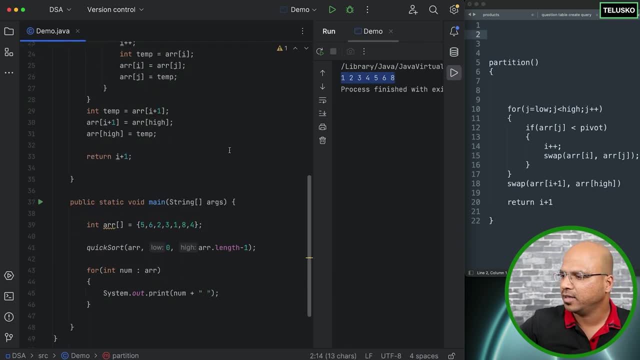